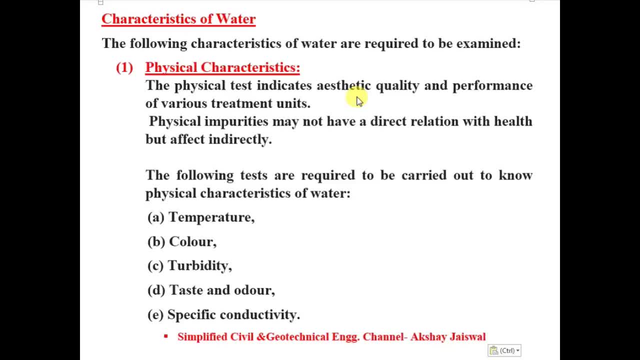 meaning if there are more impurities present in the water, then we call such water as dirty water. In other language it is called turbid water. If the water is clean and transparent, then we call such water as non-turbid water sample. 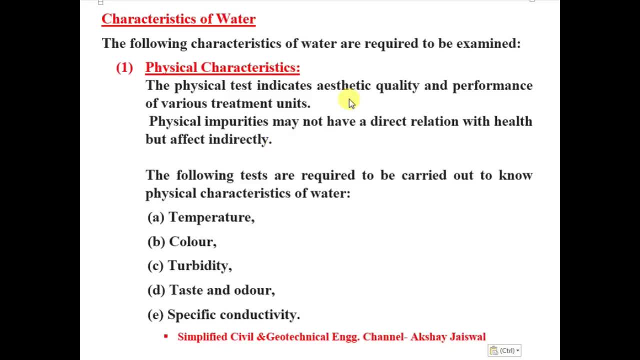 Let's see the next points. There is no direct impact of physical impurities on our health, but indirectly it will have an effect on our human health. Next point is the following: tests are required to be carried out to know the physical characteristics of water. 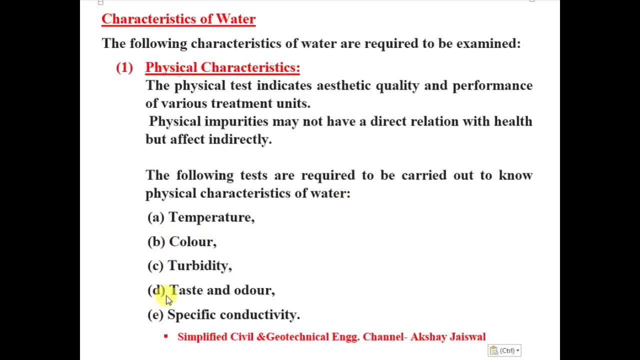 These tests are temperature, colour, turbidity, taste, odour and the last one is specific conductivity. To physically test the water we have to go down, We have to conduct some tests. For example, we have to check the temperature, colour, turbidity, taste, odour. 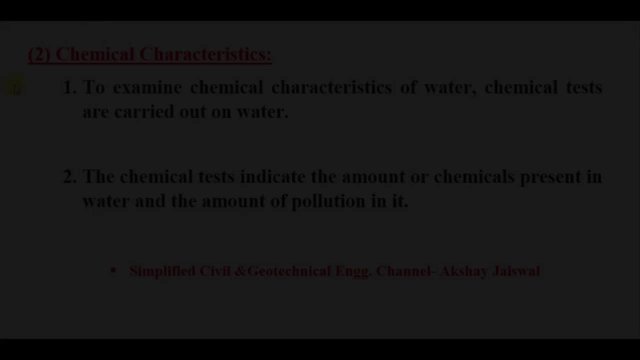 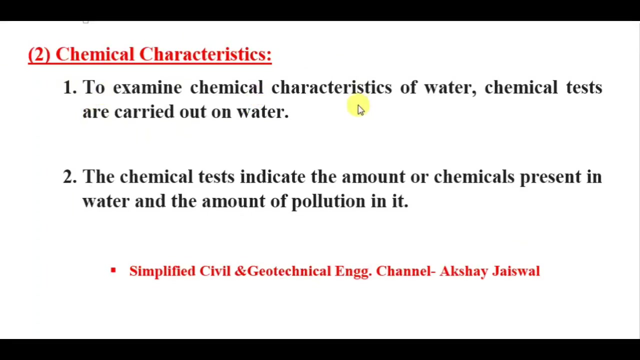 and the last one is specific conductivity. Next characteristics is chemical characteristics. First point is to examine chemical characteristics of water. chemical tests are carried out on water And second one is: the chemical tests indicate the amount or chemicals present in water and the amount of pollution in it. 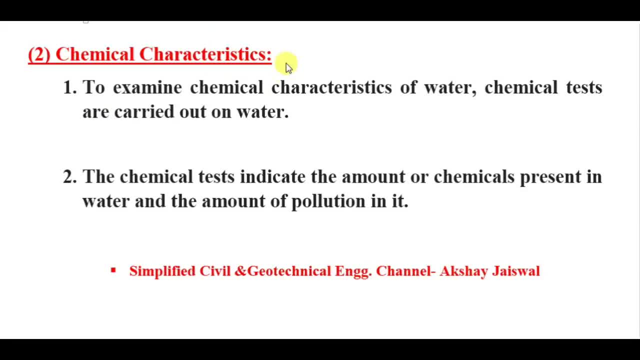 According to the name, chemical characteristics. it says that the tests which are carried out to know the chemicals which are present in water. Here, in the first point, some chemical tests are done on water. Here we get to know which types of chemicals are present in water. 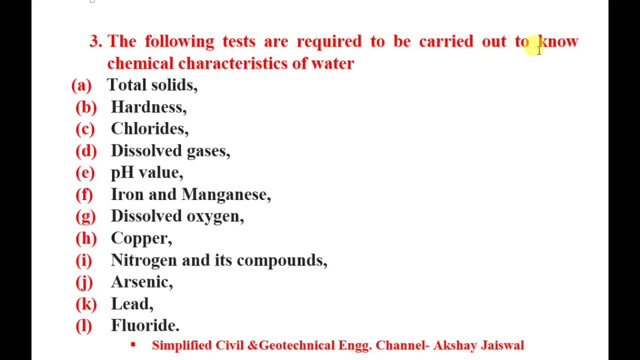 Next point is the following tests are required to be carried out to know chemical characteristics of water. First one is total solid, Second, hardness, Third, chlorides. Next one is dissolved oxygen, Then pH value, Iron and manganese. 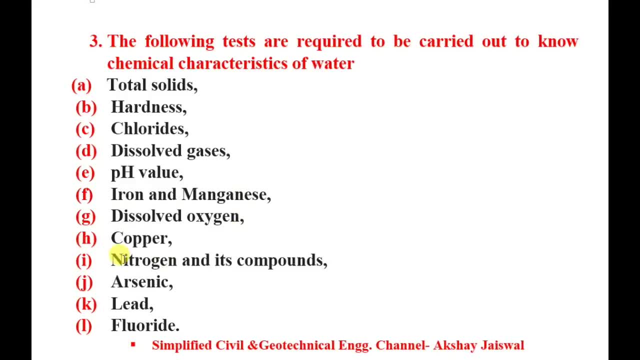 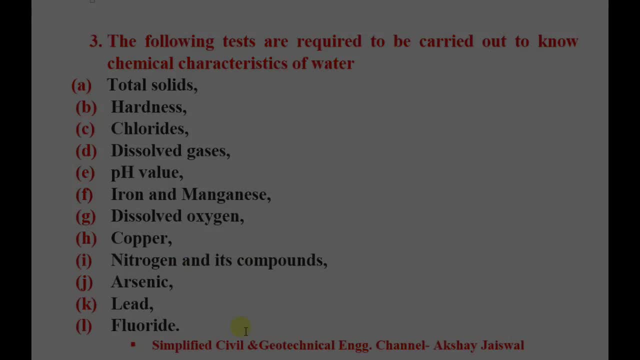 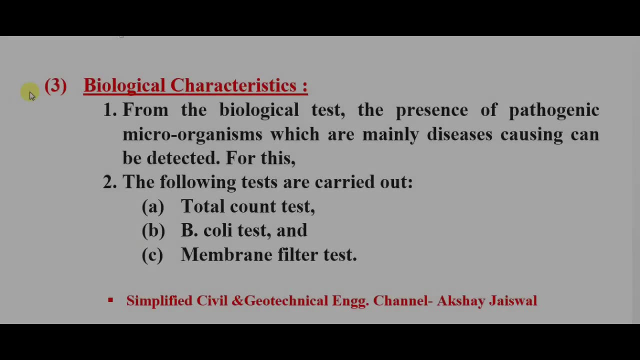 Dissolved oxygen, Copper, Nitrogen and its compounds, Arsenic, Lead, And last one is Fluoride. Now we will see third characteristics, which is biological characteristics. Point number one from the biological test: the presence of pathogenic microorganisms. 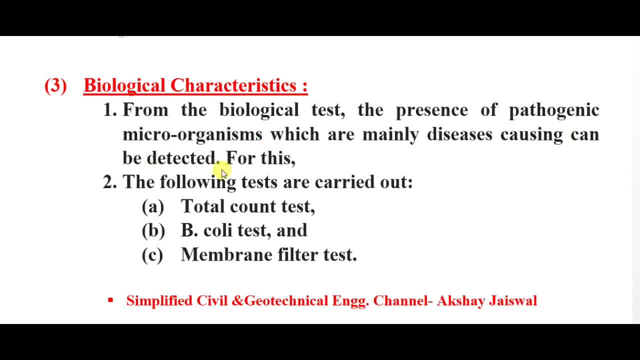 which are mainly disease causing, can be detected. For this purpose, following tests are carried out: First one is total count test, Second one is Decoli test And last one is Membrane filter test By conducting biological test. 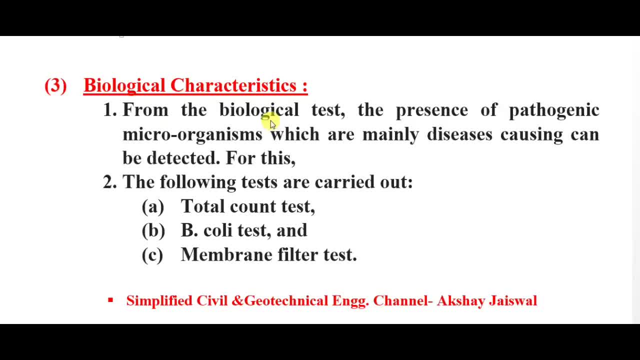 we can find out the amount of pathogenic microorganisms which are present in water And pathogenic microorganism means which can affect our human health. Those are known as pathogenic microorganisms Here. third type is biological characteristics. 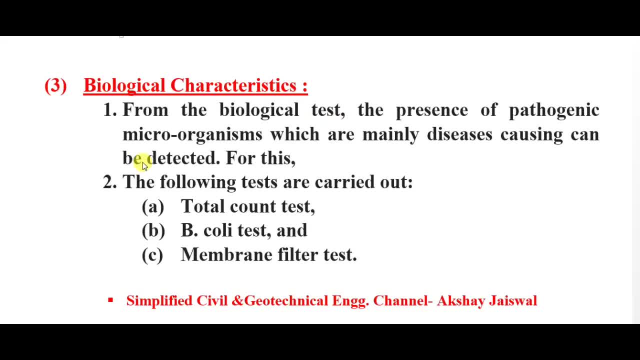 Or which we will call biological test, And after performing biological test, the pathogenic microorganisms present in water means which affects our human health, or affects our human health, which is the main reason for humans to get sick. 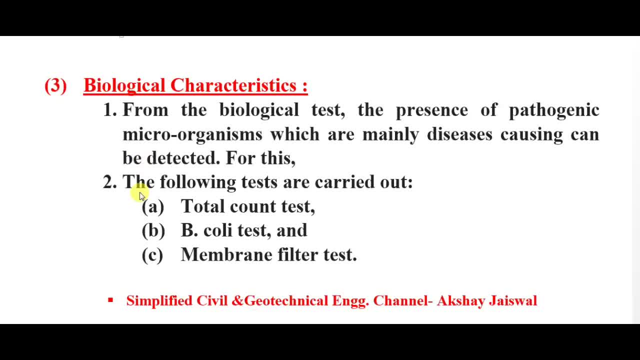 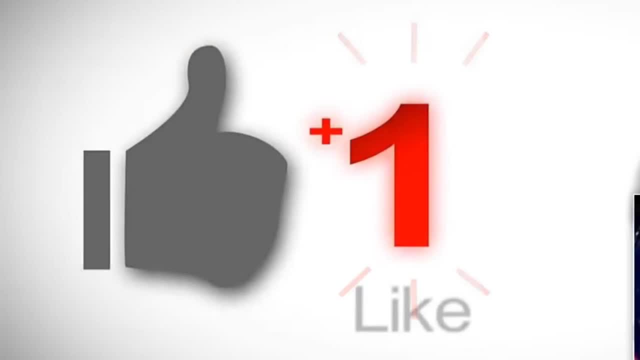 We can detect such bacteria here. In biological testing, three types of tests are taken, In which first test is total count test, Second is Decoli test And last test is Membrane filter test. Now let's see. 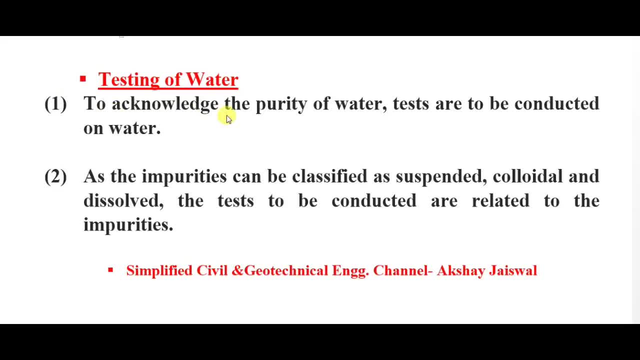 testing of water. First point is to acknowledge the purity of water. tests are to be conducted on water. Point number two, as the impurities can be classified as suspended, colloidal and dissolved, the tests to be conducted are related to the impurities. 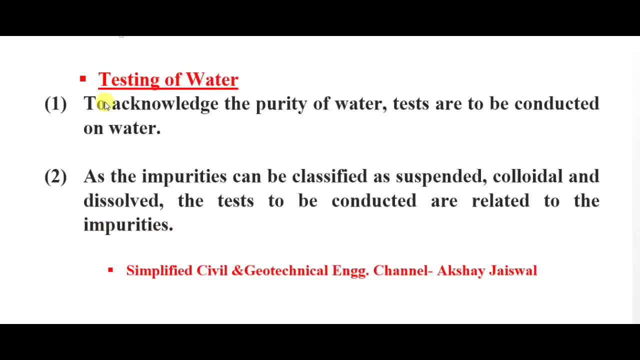 Here we are seeing testing of water. By testing of water, we get to know how pure the water is And after testing the water we get to know suspended impurities, colloidal impurities and dissolved impurities. 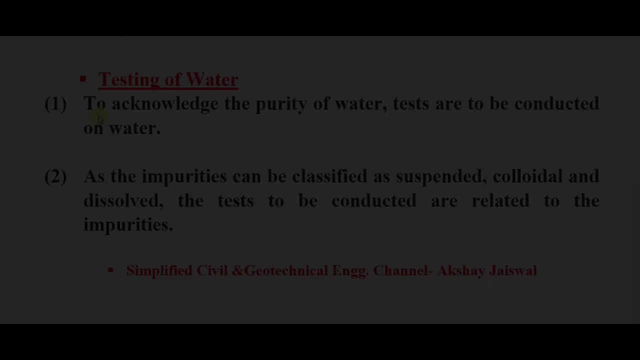 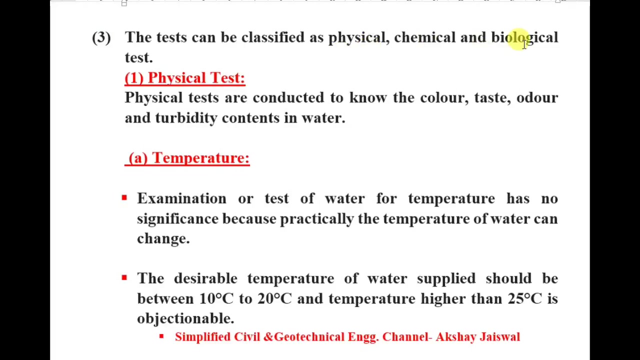 From here we get to know. Next point is the test can be classified as physical, chemical and biological test. First test is physical test. Physical tests are conducted to know the colour, taste, odour and 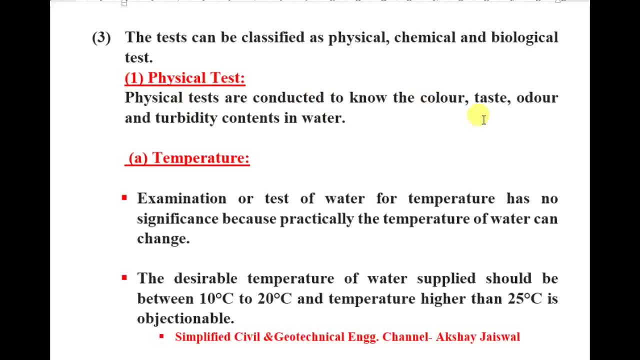 permeability contents in water. The testing of water is classified in three types: Physical, chemical and biological. First test is to know the colour, taste, odour and permeability contents in water. The first type is 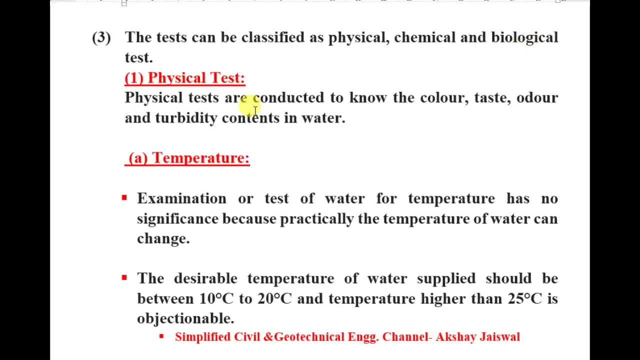 physical testing, Where colour, taste, odour and permeability contents are included in physical testing. Next point is temperature Examination or test of water, for temperature has no significance because practically 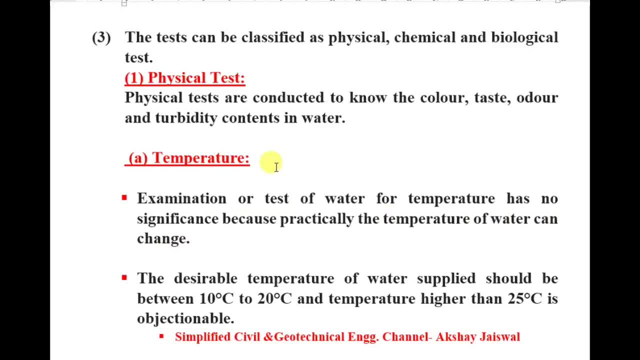 the temperature of water can change. Here the first point in testing is temperature. The importance of temperature is not that much because practically if we see the temperature, the temperature can rise, or the temperature 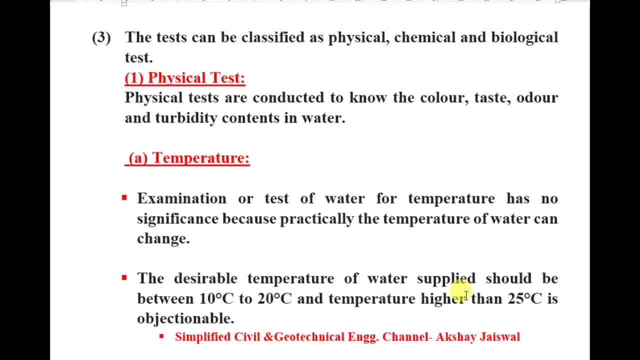 can fall. Next point is the desirable temperature of water supplied should be between 10 to 20 degree centigrade, and temperature higher than 25 degree centigrade is objectionable. Generally, the temperature of water 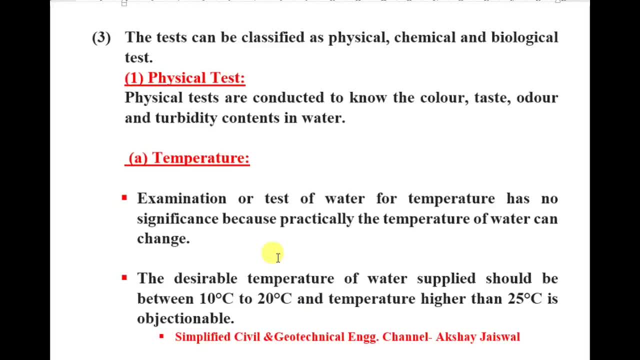 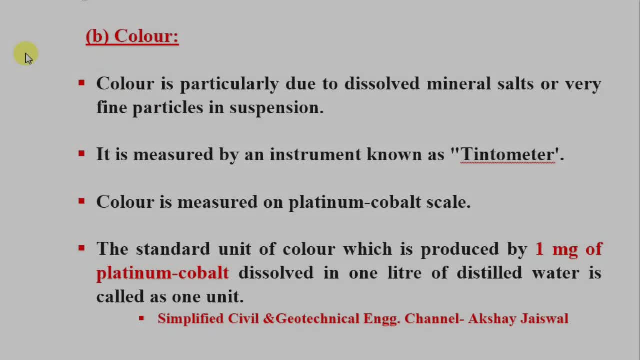 should be between 10 to 20 degree. If the temperature of water is above 25 degree, this type of water is considered objectionable. Next physical test is color. First point is color is particularly. 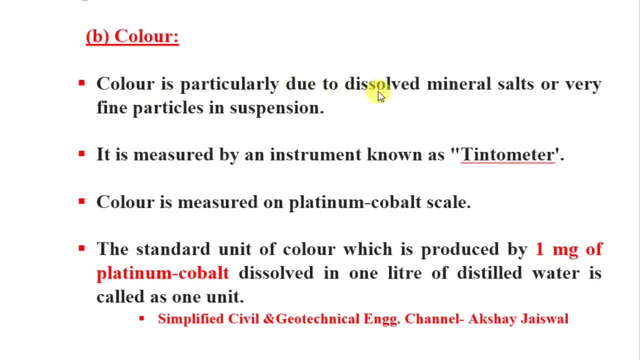 due to dissolved mineral salts or very fine particles in suspension. It is measured by an instrument known as tintometer. Color is measured on platinum cobalt scale. and last one point is the standard unit of color. 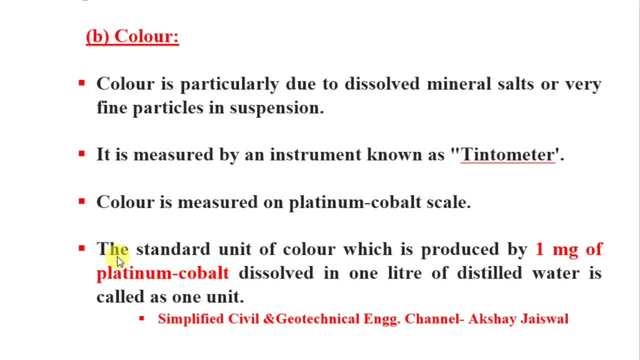 which is produced by the temperature of water and temperature. It is measured by 1 milligram of platinum cobalt dissolved in 1 liter of distilled water. It is called as: 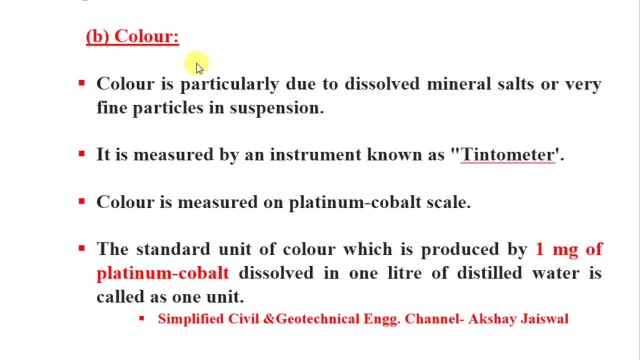 1 milliliter Here. our second type of physical testing is color. Color is particularly due to dissolved mineral salts. The main reason for changing the color of water is dissolved salts, or 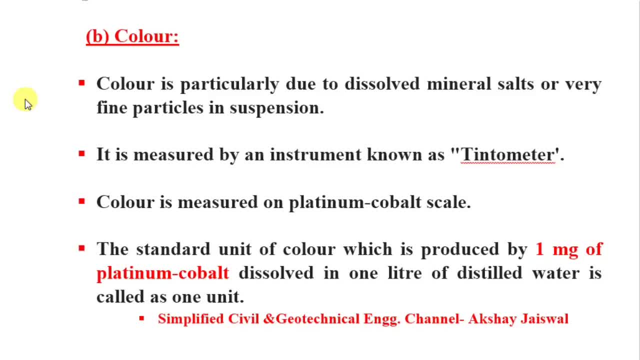 or another reason is to measure color. we use this instrument, the color meter, To measure color. the instrument which is used is called Tintometer And the scale to measure color is the platinum cobalt scale. 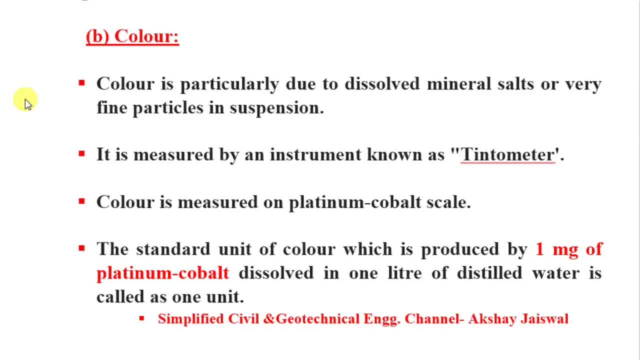 And the last point is the standard unit. The standard unit of color is this way: For example, 1 milligram of platinum cobalt in 1 liter of distilled water, after dissolved in. 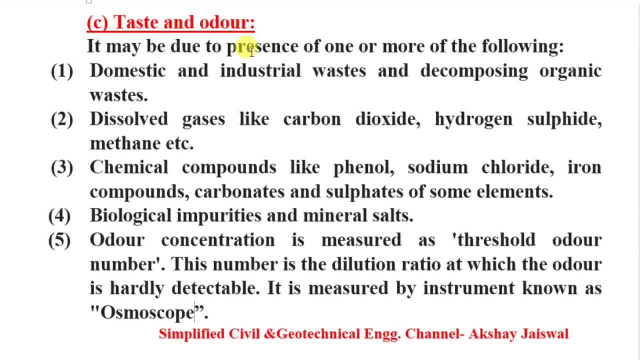 this color is and order. it may be due to presence of one or more of the following: first point is domestic and industrial waste and decomposing organic waste. second point is it is due to dissolved gases like carbon dioxide, hydrogen sulfide and methane. third test and order is produced due to chemical compounds like phenol. 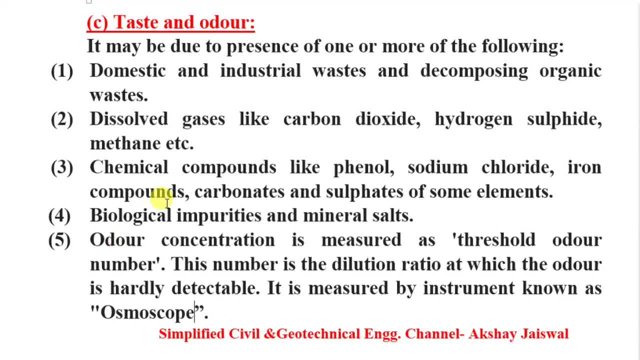 sodium chloride, iron carbonates and sulfates of some elements, point number 4, that is, biological impurities and mineral salts. and point number 5: order concentration is measured as threshold order number. this number is the dilution ratio at which the order is hardly detectable, and it is measured by the 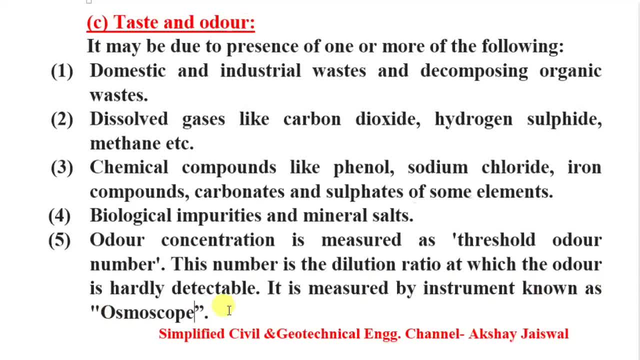 instrument known as osmosis. next point is test and order. if there is no proper water test and there is any bad smell, first is domestic and industrial waste. second reason is presence of dissolved gases like carbon dioxide, hydrogen sulfide and methane gas. third reason is this: chemical compounds. 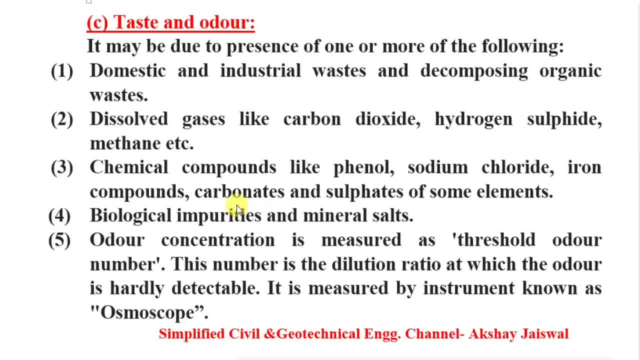 like phenol and sodium chlorideụcde. and to the second reason is we have homeostatic Odium Chloride, Iron Compounds, Carbon X and Sulfates of some elements. Fourth reason is Biological impurities, ie presence of bacteria or mineral salts. 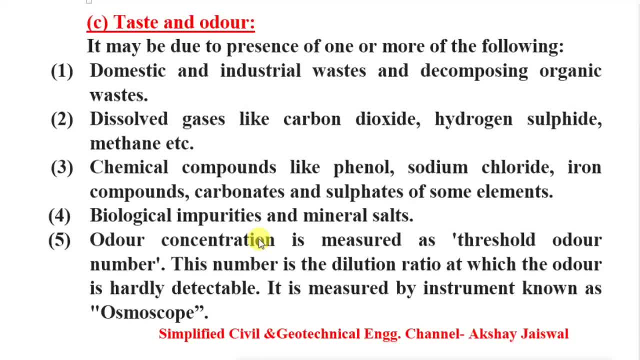 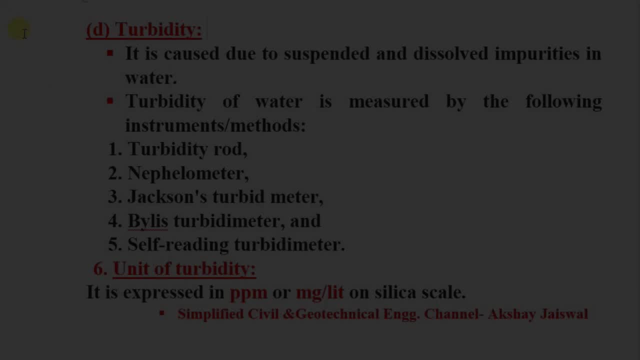 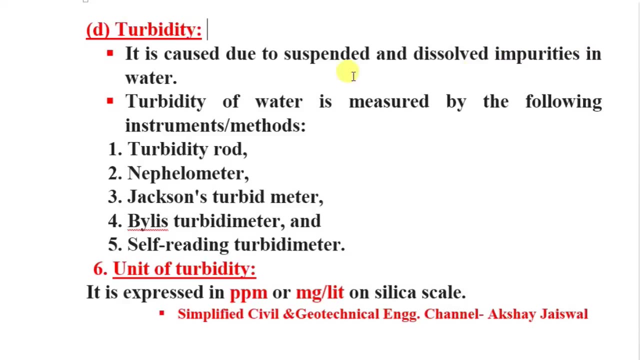 Mineral salts are also a reason due to which bad smell can be produced. Order concentration is measured by threshold number. This number is dilution ratio. The instrument used to measure this is Osmoscope. Next physical characteristic is Turbidity. It is caused due to suspended and dissolved impurities in water. 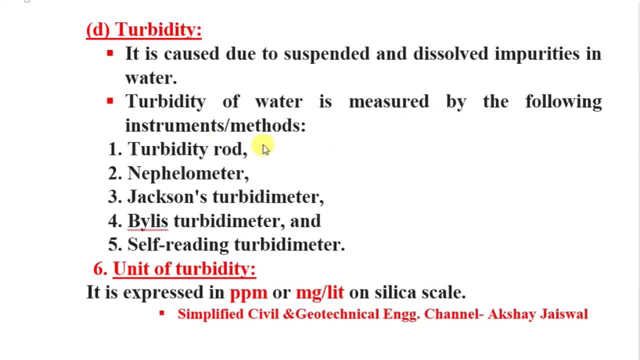 Turbidity of water is measured by following instruments: First one is Turbidity Rod, Second one is Nephiloid, Third one is Jackson's Turbidity Meter, Fourth one is Bailey's Turbidity Meter And last one is Self Reading Turbidity Meter. 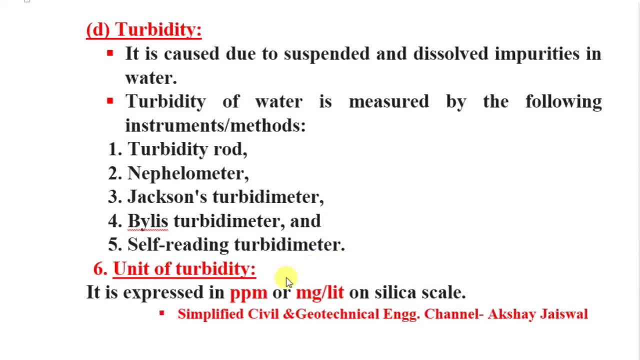 Now we will see unit of turbidity. It is expressed in ppm, ie parts per million, Or another unit is mg per liter on silica scale. As it is already discussed, Turbidity of water is measured by. Turbidity is one kind of transparency of water. 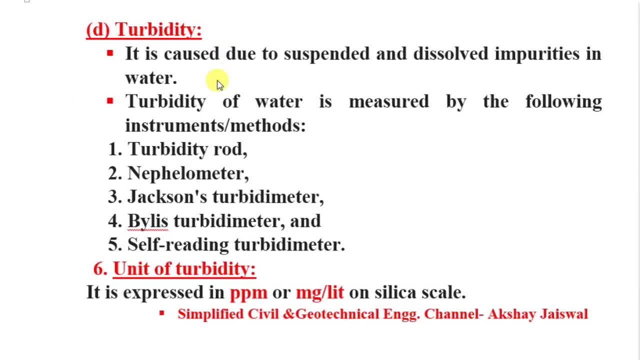 More the turbid water, then we can say more the impurities are present in water. If water is transparent, then we can say that it is non-turbid solution. Turbidity means the transparency of water is reduced due to impurities present in water Means. if water is completely clear, then we can see it from one side to another side. 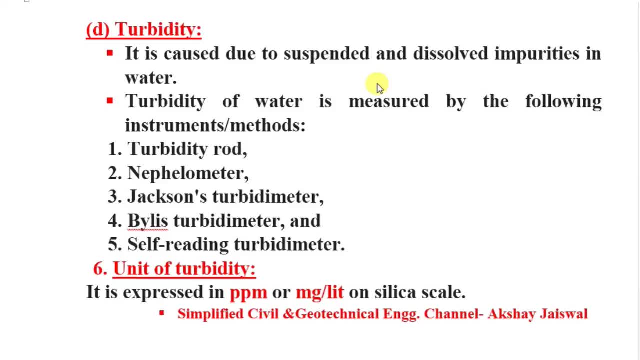 But if some impurities are present in water- For example if there are some chemical impurities present in water, Then the colour of water will change. And if we see from the other side of water, then we will not see anything. So we will call such water as Dirty Water. 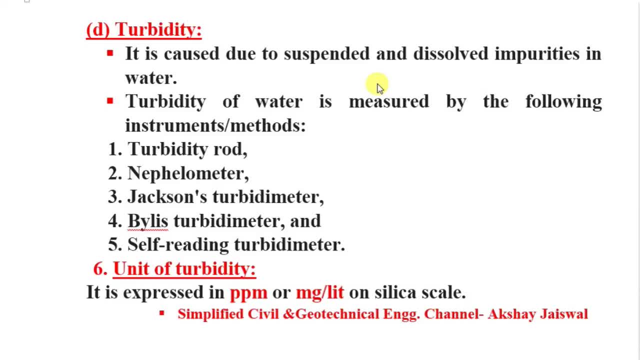 Which will have some or the other turbidity value, And the water which is not clear, We will call it as Turbid Water. And there are some instruments to measure turbidity, Which are Turbidity Meter, Nephiloid Meter, Jackson's Turbidity Meter, Bailey's Turbidity Meter and Self Reading Turbidity Meter. 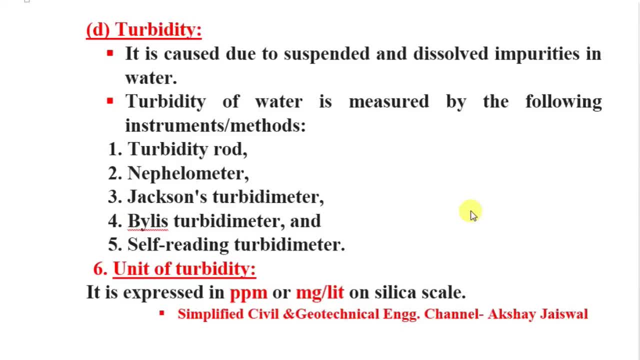 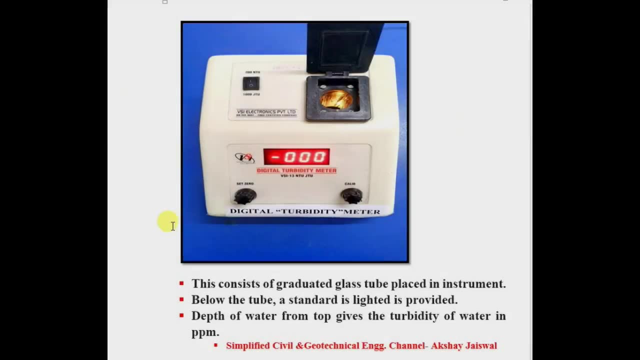 To express the turbidity. the two units are like this: First is Parts Per Million ie PPM And the second unit is MG Per Liter- ie Milligram Per Liter on Silica Scale. In this figure we can see Digital Turbidity Meter. 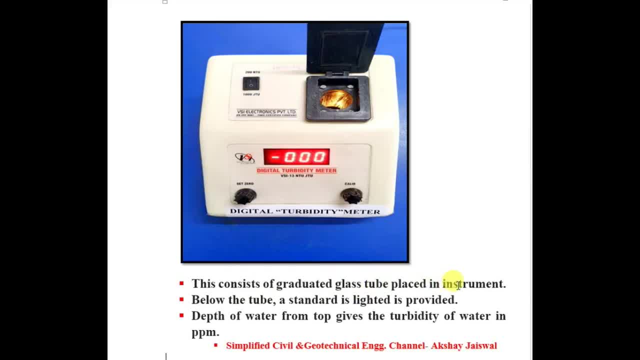 This consists of graduated glass tube placed in instrument. Here we can place glass tube Below the tube. a standard light is provided. We can see light which is reflecting from this place And depth of water from top gives the turbidity of water in PPM. Here you can see Digital Turbidity Meter.